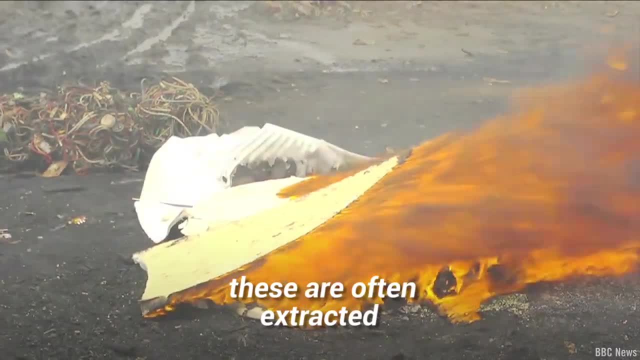 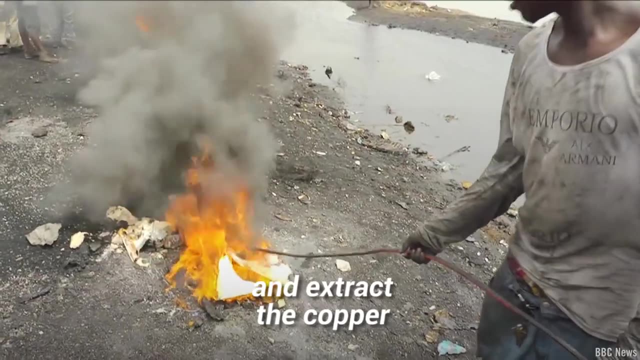 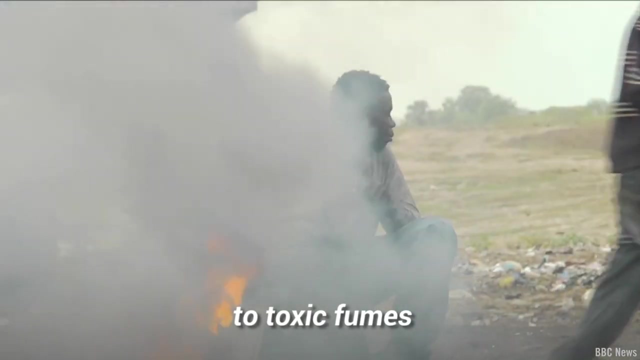 such as copper and gold. However, these are often extracted using fairly primitive methods such as burning cables to remove the plastic and extract the lead. These methods expose workers, who are often children, to toxic fumes. According to the WHO, several organizations have highlighted the need for interventions. 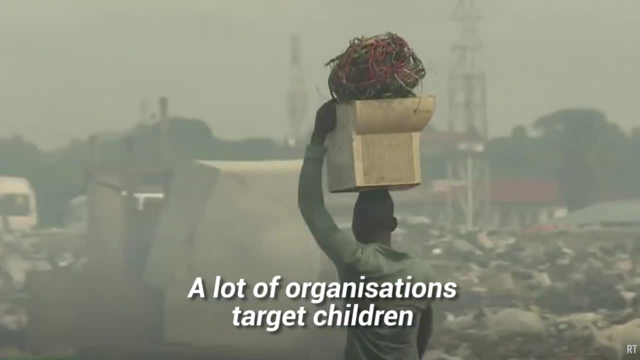 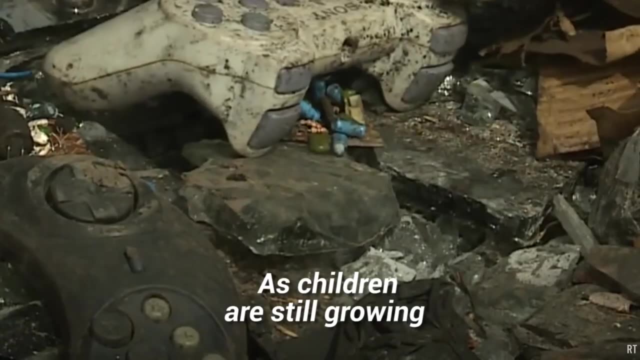 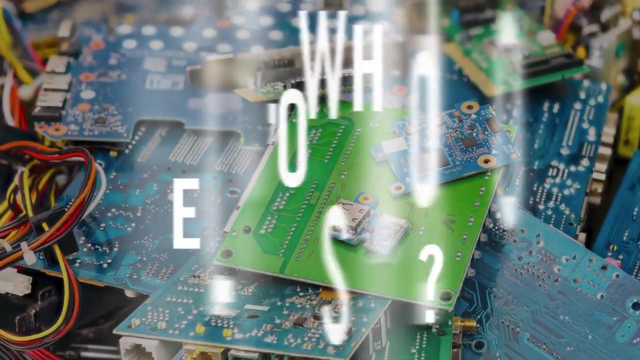 in the field of e-waste. A lot of these organizations target children, as they are the most vulnerable to harm from exposure to e-waste. As children are still growing, harmful substances can affect their development to a greater extent. So what can you do to help combat e-waste? 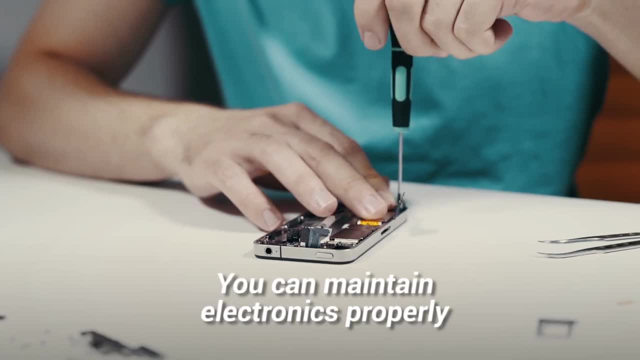 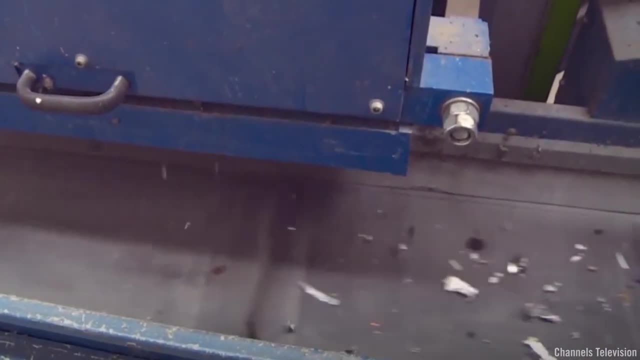 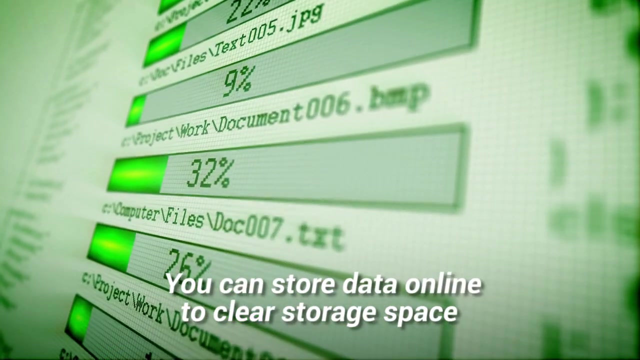 You can sell or donate old electronics. You can maintain electronics properly so they last longer. You can recycle and dispose of e-waste properly. Before buying a new electronic device, consider repurposing an old one. You can store data online to clear storage space and help your electronics last longer. 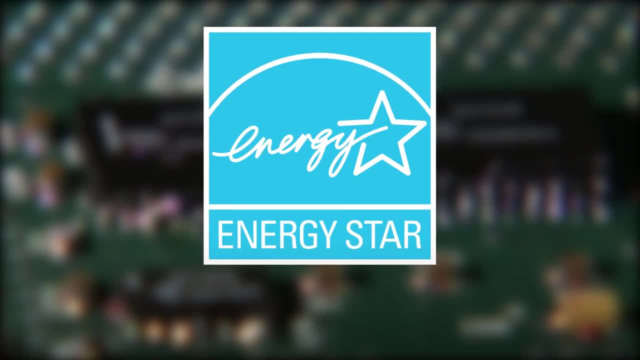 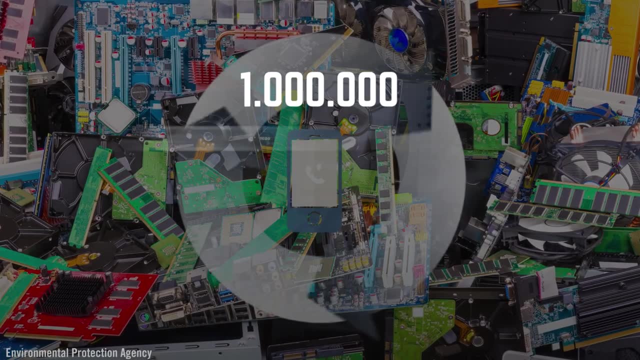 You can buy ENERGY STAR rated electronics. You can buy ENERGY STAR rated electronics. You can buy ENERGY STAR rated electronics. There is good reason to follow these few simple rules By recycling one million cellphones, more than 35 thousand pounds of copper, 33 pounds. 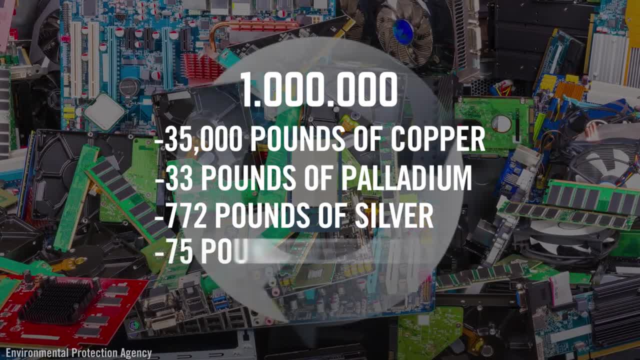 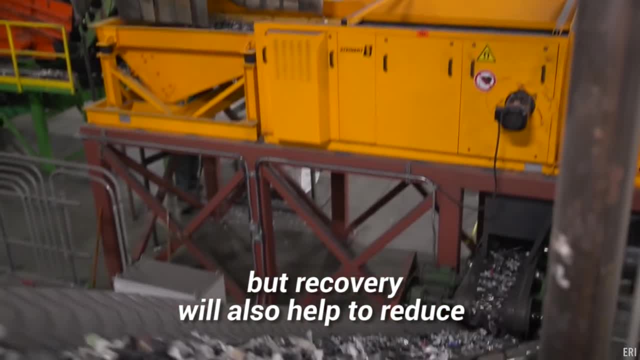 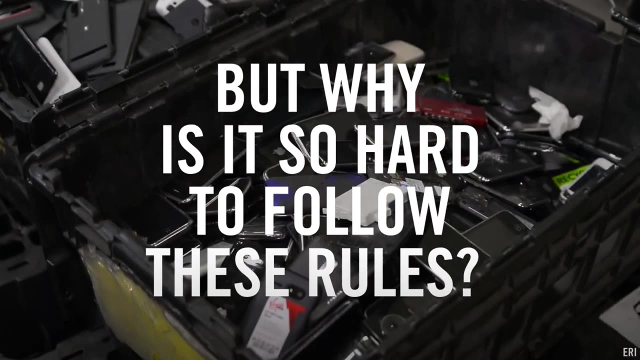 of palladium, 772 pounds of silver and 75 pounds of gold can be recovered. That material is not only worth money, but recovery will also help to reduce the amount of mining necessary. But why is it so hard to follow these rules? I'll explain, Because nowadays are made to be replaced, It's called planned obsolescence. Take, for example, how Apple's latest operating system made extensive use of haptic features that required an iPhone 6s and so forth. These kinds of features are very common in today's electronics, and so you are. 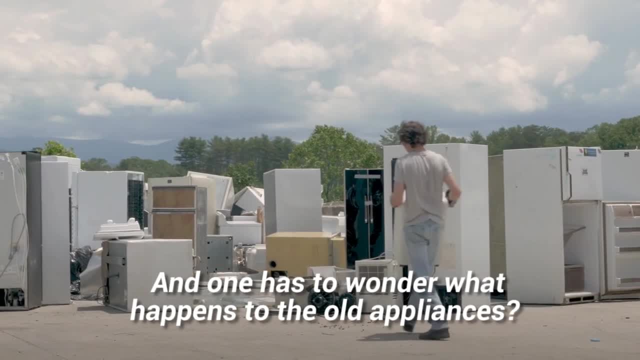 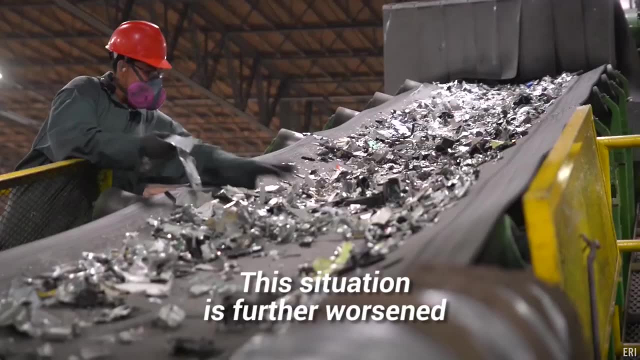 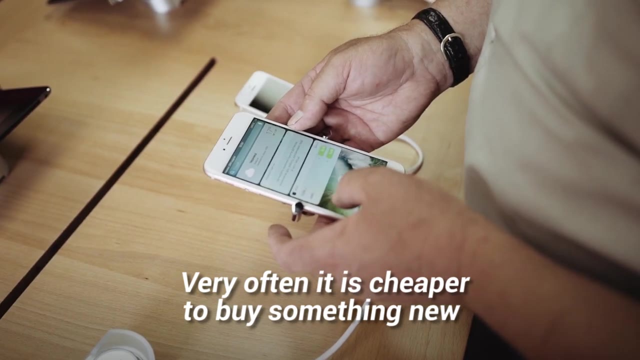 forced to replace them, And one has to wonder what happens to the old appliances? Can they be fully recycled now that parts of them are no longer needed? This situation is further worsened by the economics of gadgets. Very often it is cheaper to buy something new than to fix something old. 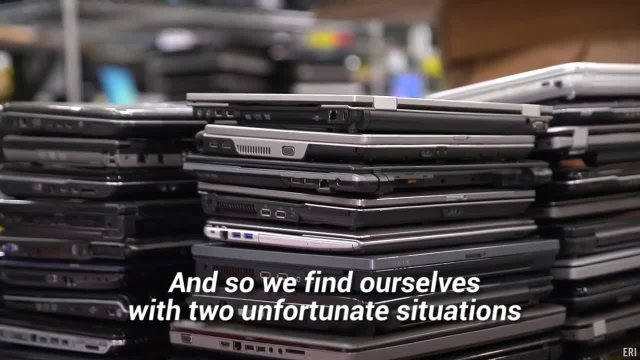 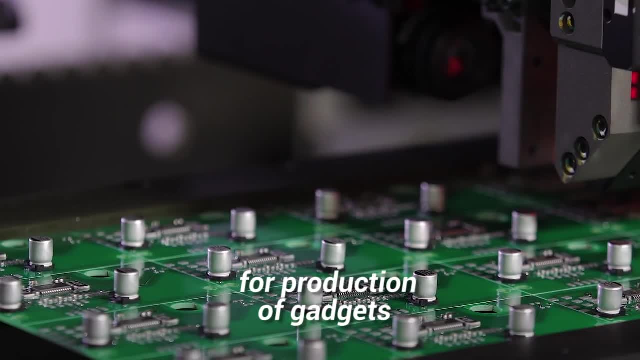 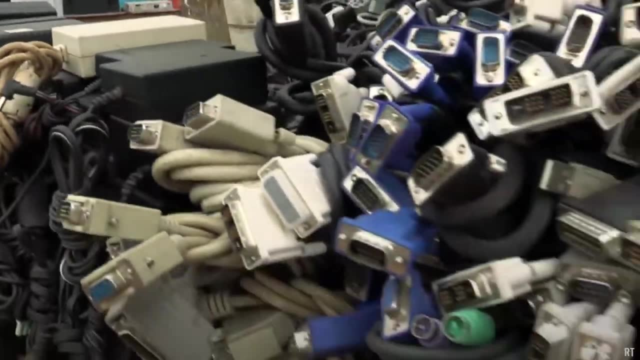 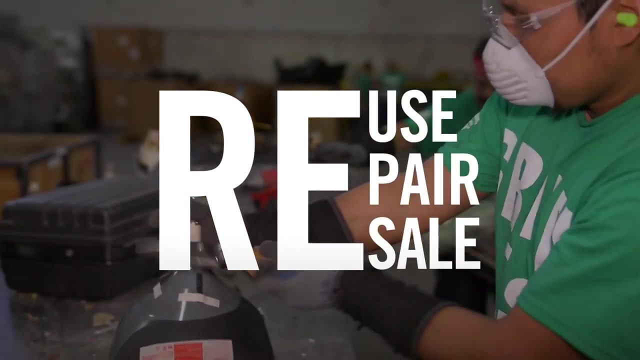 and so we find ourselves with two unfortunate situations. The first is the dangerous increase in mining for procurement for the materials needed for production of gadgets, And the second is large amounts of electronics in landfills leaking toxicity. What is sad is that this waste could easily be reduced by reuse, repair or resale.